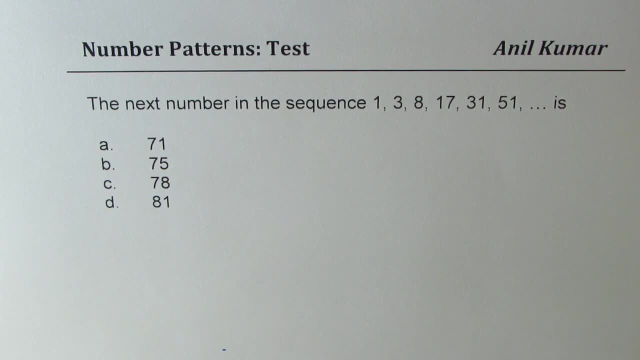 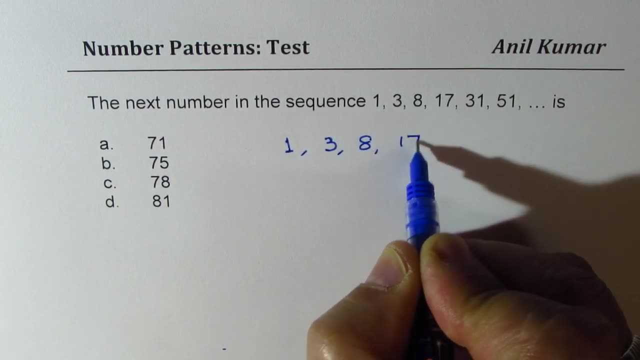 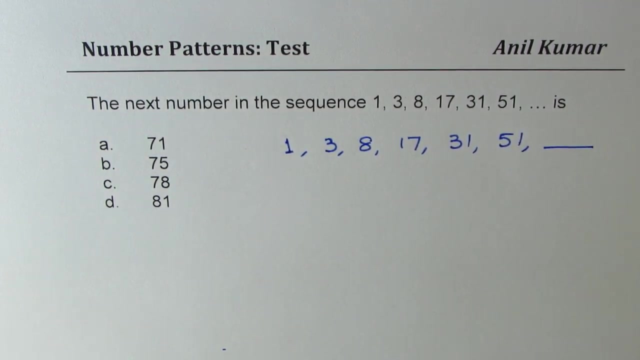 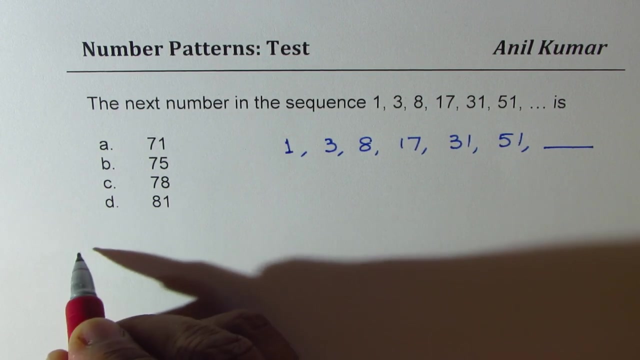 Now, this is not a very simple sequence. Let's try to work it out. So the numbers given to us are 1, 3, 8, 17, 31 and 51. We need to find the next number right. So the strategy here is to find the common difference That can give us some idea. So 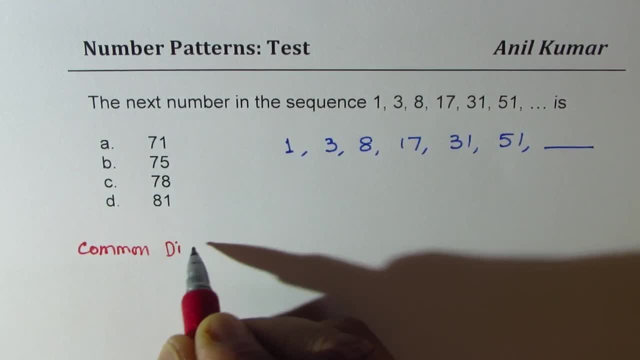 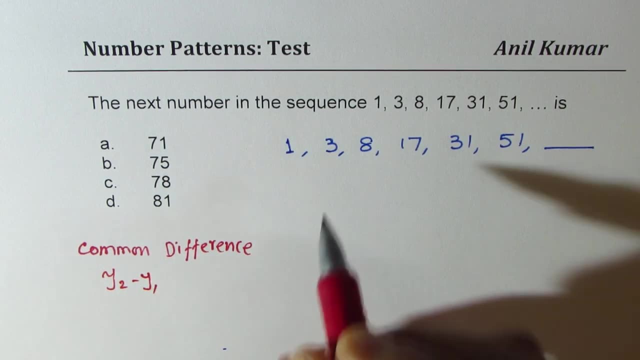 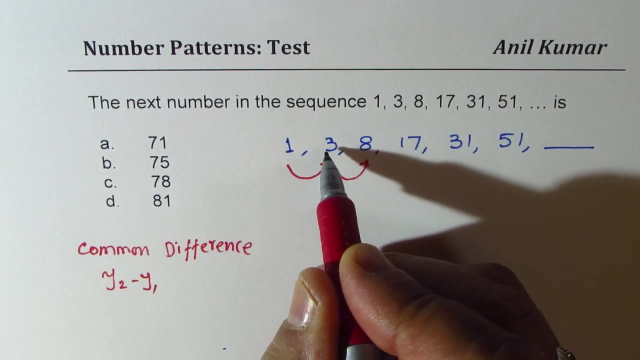 we need to find the common difference to solve such questions. Now, common difference is kind of y2 minus y1.. So what we will do here is we'll find what is the value of 3 minus 1 and what is the value of 8 minus 3 and then check the pattern. Now, 3 minus 1 is 2,. 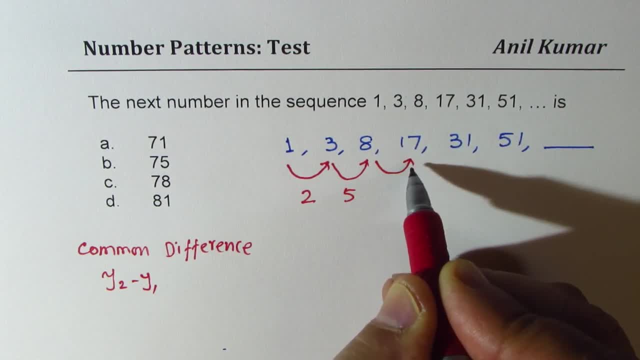 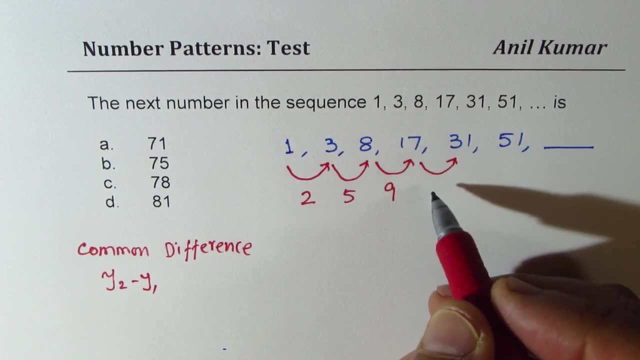 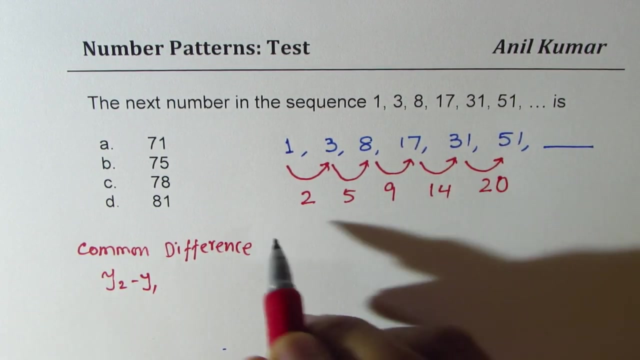 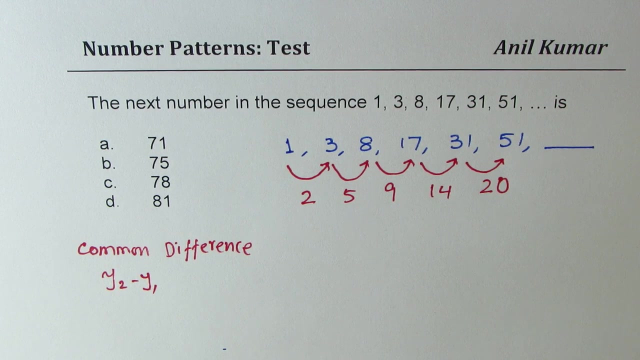 8 minus 3 is 5 and 17 minus 8 is 9, 31 minus 17 is 14 and 51 minus 31 is 20.. So we kind of get this common difference now: 2, 5, 9, 14, 20 really does not give you any pattern. so 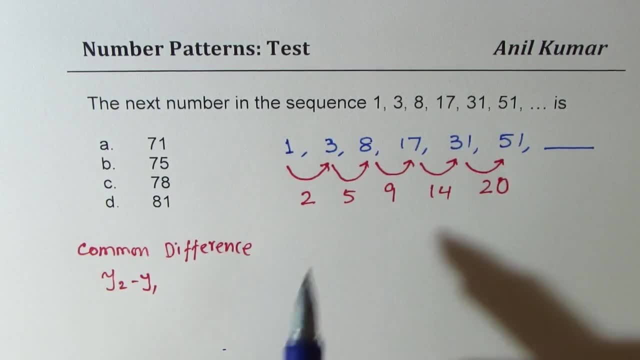 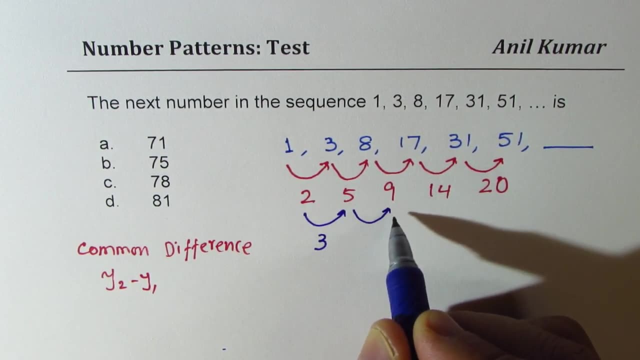 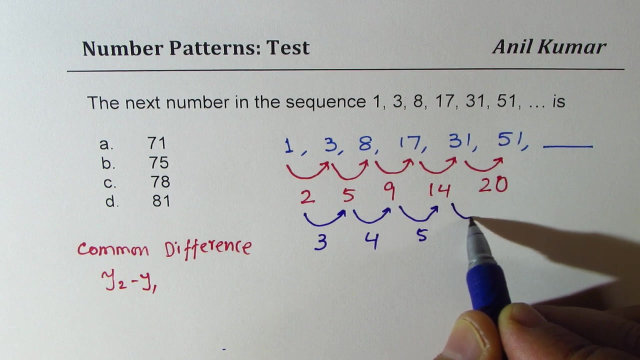 let's find the next common difference. okay, so we'll find the next common difference, which is 5 minus 2, which is 3, and then we'll do 9 minus 5, which is 4. 14 minus 9 gives us 5. 20 minus 14 is 6. now that is the pattern you can see now. 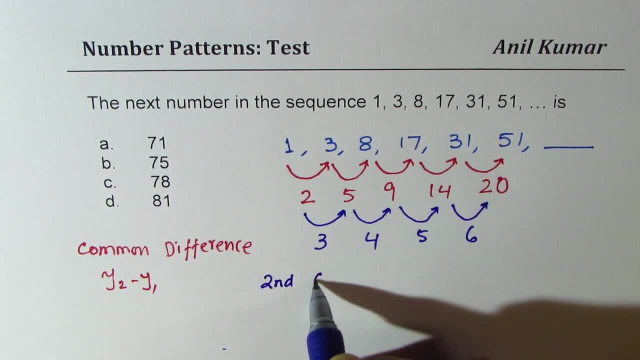 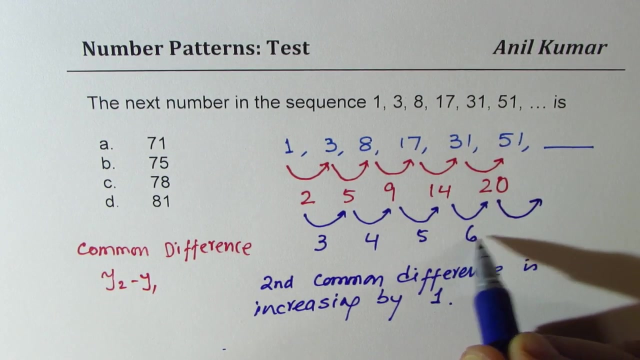 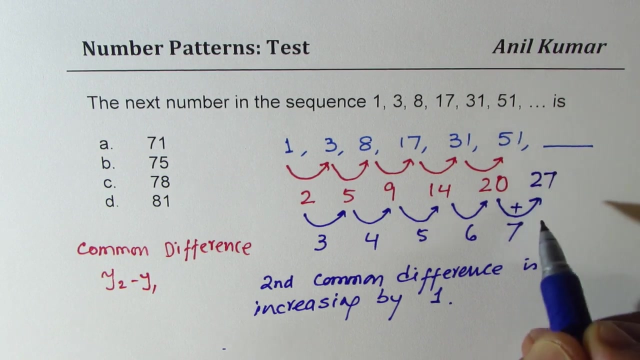 right. so what do you notice here is that the second common difference is increasing by 1 now, knowing that we know for the next number, the common difference should be 7 right now. if that is the case, then adding 7 to 20 will give us 27, and now? 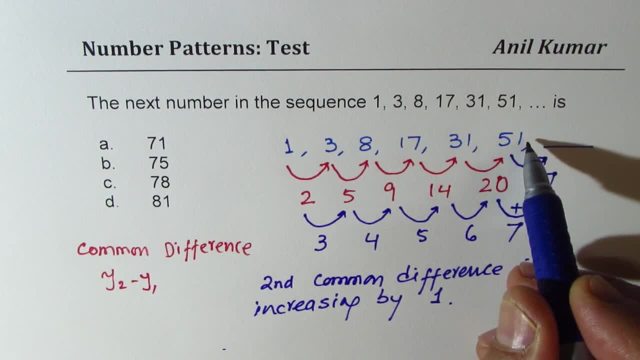 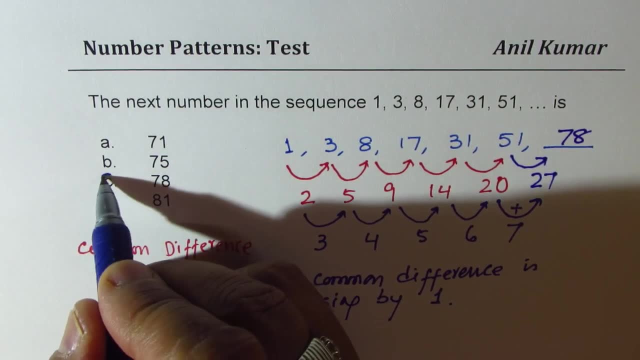 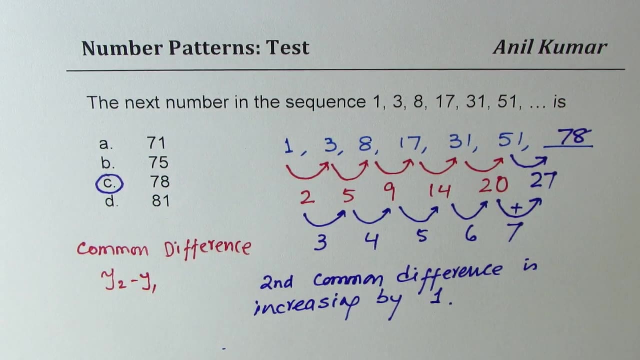 adding 27 to 51 gives us the next number correct, so which becomes 78. do you see that? so option C is the right option. perfect, so you can see how we can actually solve such questions. so that is a very important question. from test point of view, feel free to write your. 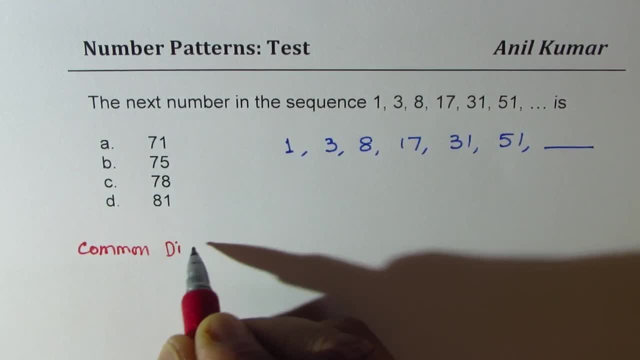 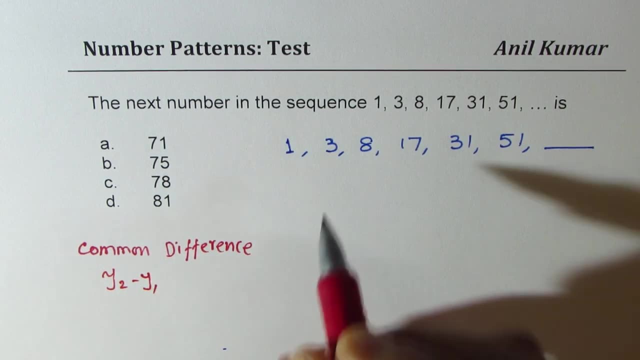 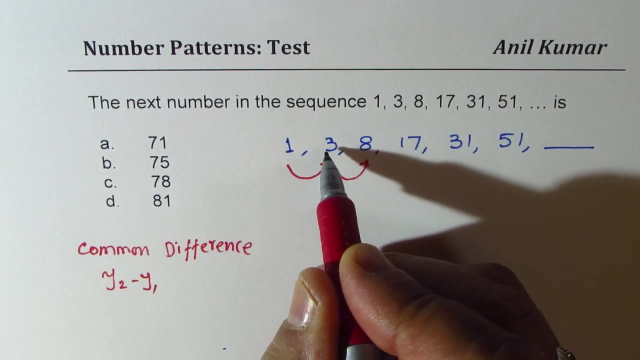 we need to find the common difference to solve such questions. Now, common difference is kind of y2 minus y1.. So what we will do here is we'll find what is the value of 3 minus 1 and what is the value of 8 minus 3 and then check the pattern. Now, 3 minus 1 is 2,. 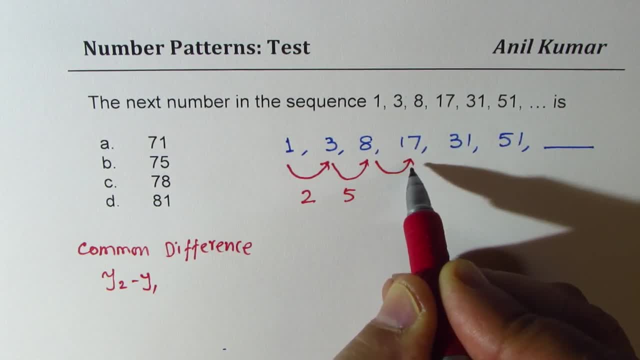 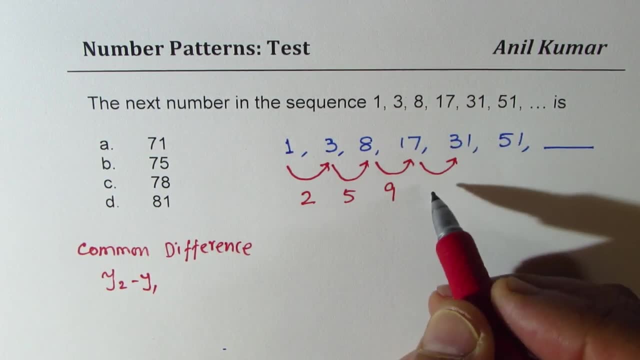 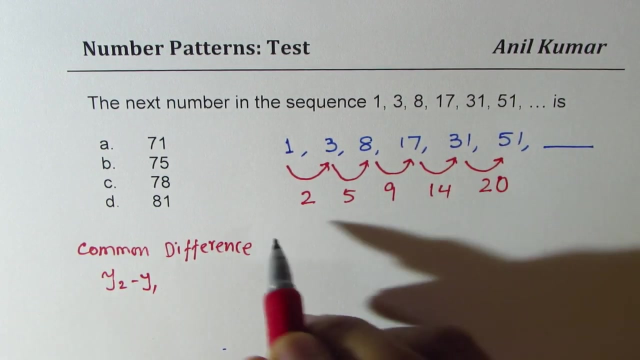 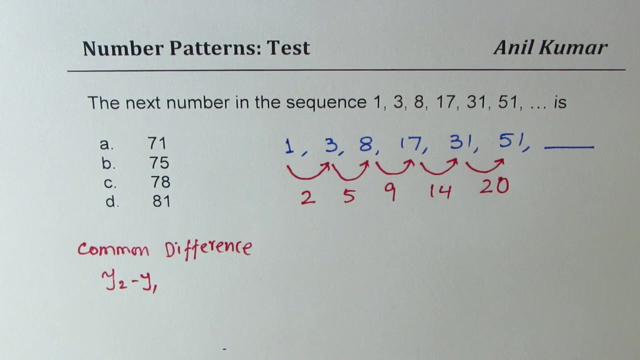 8 minus 3 is 5 and 17 minus 8 is 9.. 31 minus 17 is 14 and 51 minus 31 is 20.. So we kind of get this common difference Now: 2, 5, 9, 14, 20 really does not give you any pattern, So let's find the. 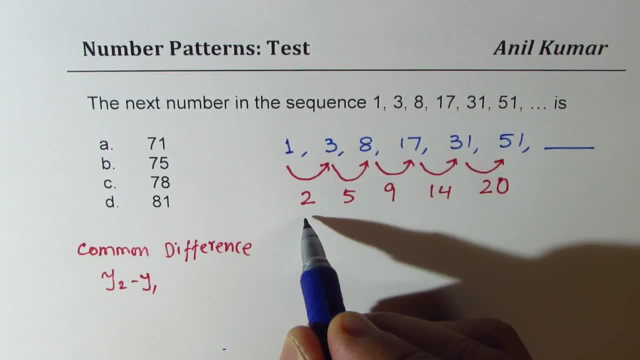 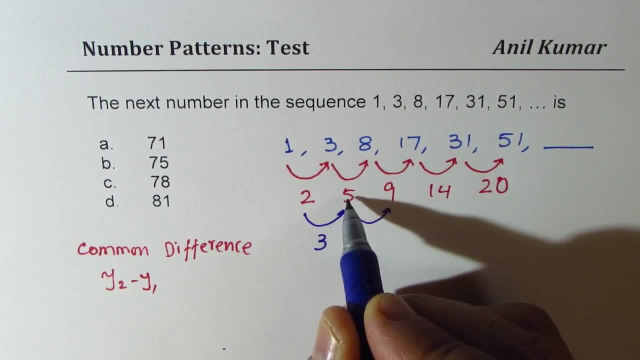 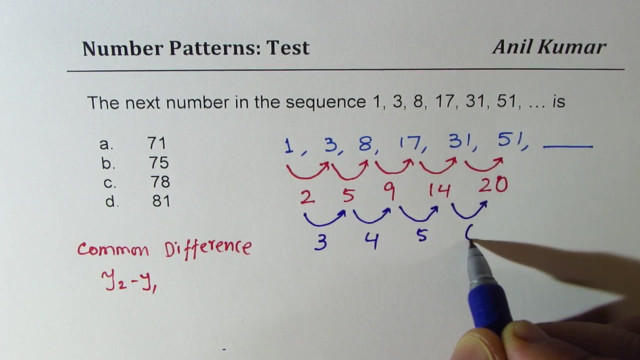 next common difference. Okay, so we'll find the next common difference, which is 5 minus 2, which is 3, and then we'll do 9 minus 5, which is 4.. 14 minus 9 gives us 5.. 20 minus 14 is 6.. 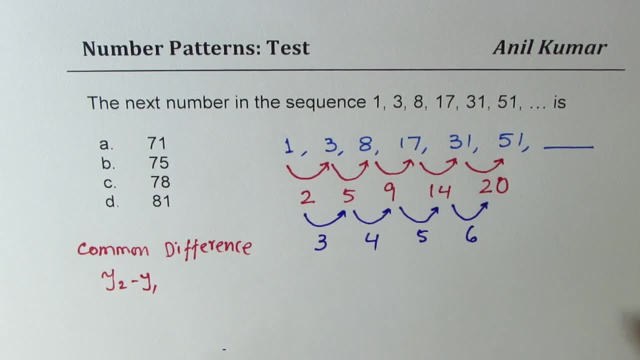 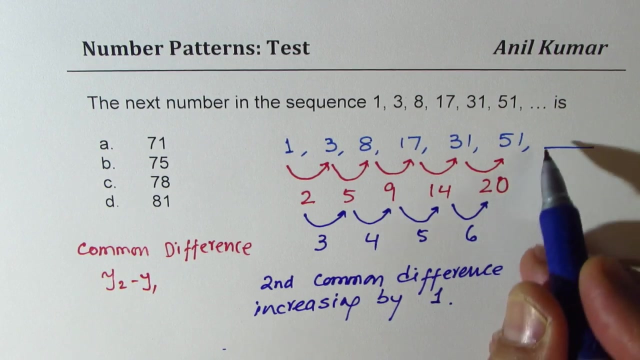 Now, that is the pattern you can see now, right? So what we notice here is that the second common difference is increasing by 1.. Now, knowing that, we know for the next number the common difference should be 7, right Now. if that is the case, then adding 7 to 20 will give us 27.. And now adding: 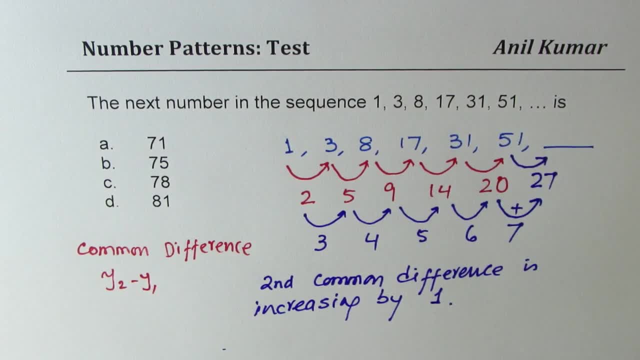 27 to 51 gives us the next number correct So, which becomes 78.. Do you see that? So option C is the right option. Perfect, So you can see how we can actually solve such questions. So that is a very important question from test point of view, Feel. 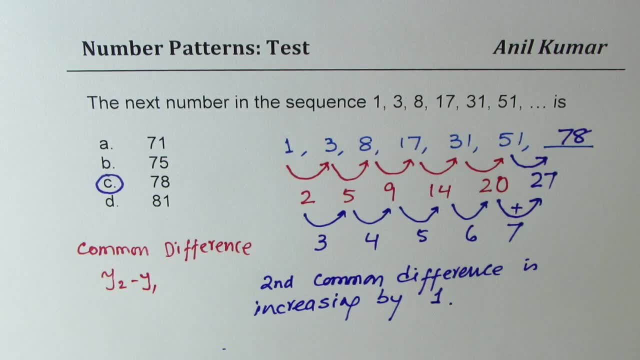 Feel free to write your comments and share your views and try to understand the strategy which we have followed here to solve such questions. Thanks for watching and all the best.